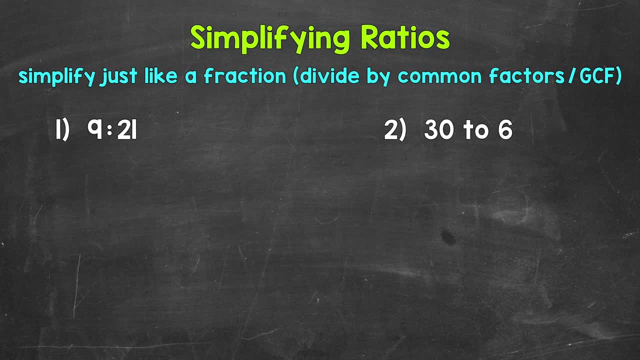 word two: I'm actually going to take our ratio and rewrite it in fractional form, So it's just like simplifying a fraction. So we have nine to twenty-one. Now we need to think about how to write a ratio in lowest terms. So let's jump into number one. 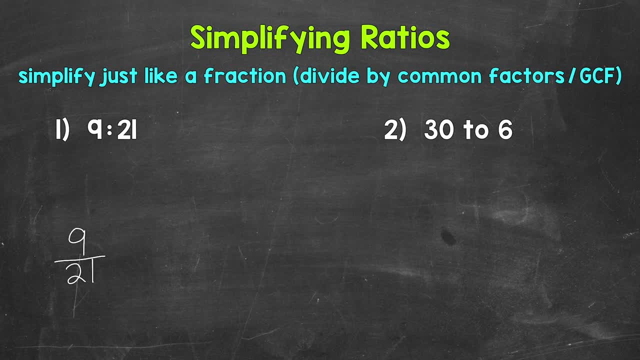 and think of common factors between nine and twenty-one Numbers that we can divide both nine and twenty-one by. Well, three is a common factor and it happens to be the greatest common factor, the largest number in value that we can divide both nine and twenty-one by. So let's divide nine. 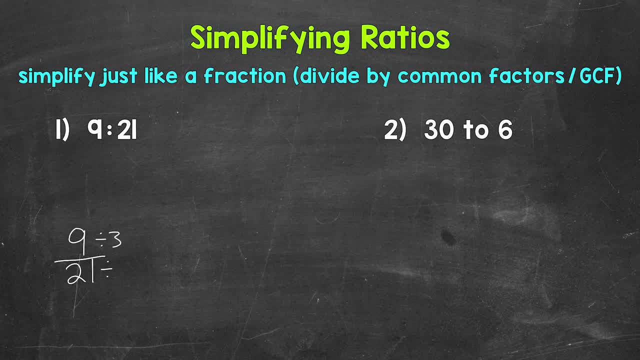 by three and twenty-one by three. Nine divided by three is three, and twenty-one divided by three is seven. so we get three to seven. The greatest common factor between three and seven is one. so we are in simplest form. Three to seven is our simplified 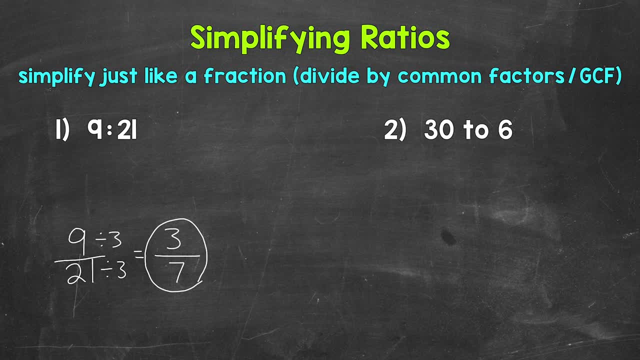 ratio. Now, like I mentioned earlier, you can simplify from the original form of a ratio. so, however, it is originally written. So, before moving on to number two, I do want to show you that we can divide both the nine and twenty-one by three, and then we get three to seven. So let's. 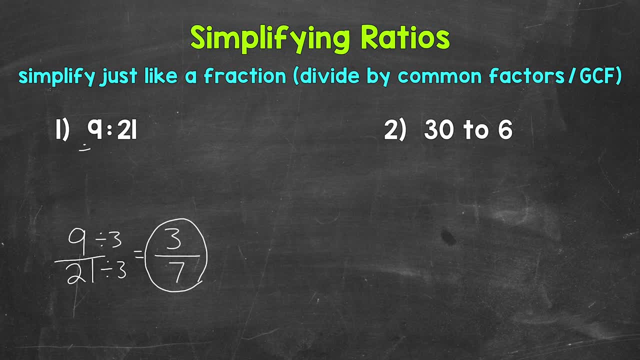 and 21 by 3 up here as well. so divide by 3, divide by 3 and we get 3, 2, 7 that way as well. now we can also take the fractional form of our simplified ratio and rewrite it using a colon: 3, 2, 7 or using the word 2. all of those ratios. 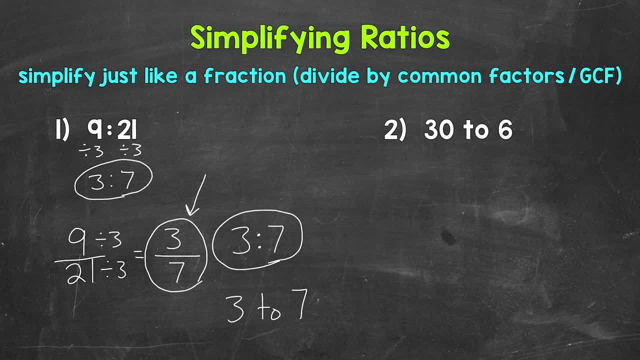 mean the same thing. so 3: 2 7 or 3 2 7. let's move on to number 2, where we have 30 to 6. I'll rewrite this ratio as a fraction as well. so 30 to 6. now we need. 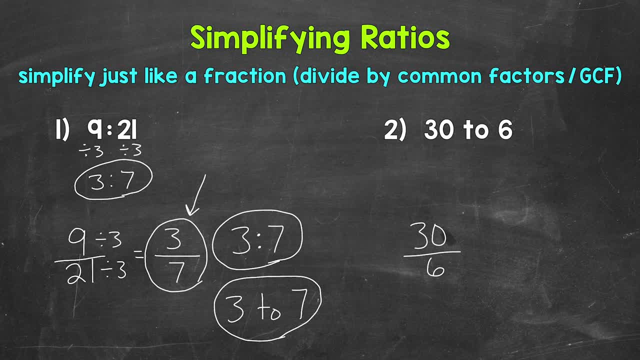 to think of common factors between 30 and 6. I'm going to start by using the greatest common factor and simplify this ratio in one way or another. so I'm going to start by using the greatest common factor and simplify this ratio in one way or another. 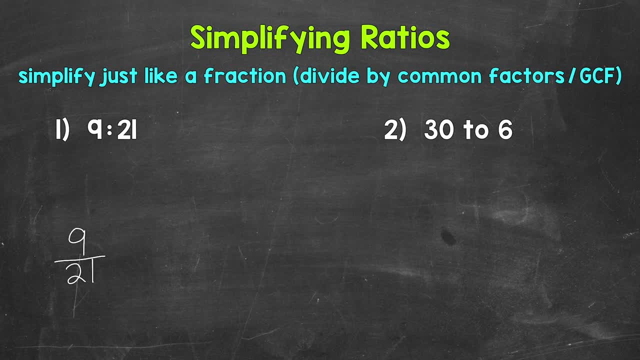 and think of common factors between nine and twenty-one Numbers that we can divide both nine and twenty-one by. Well, three is a common factor and it happens to be the greatest common factor, the largest number in value that we can divide both nine and twenty-one by. So let's divide nine. 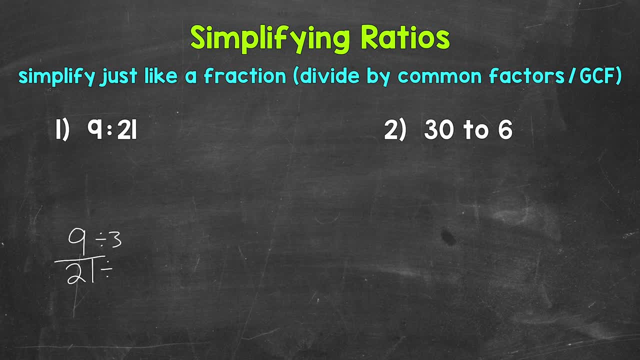 by three and twenty-one by three. Nine divided by three is three, and twenty-one divided by three is seven. So we get three to seven. The greatest common factor between three and seven is one. So we are in simplest form. Three to seven is our simplified 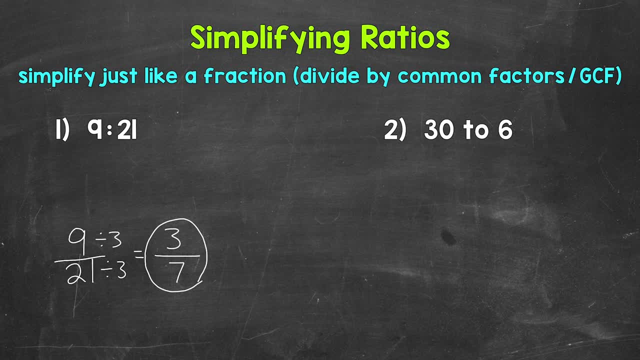 ratio. Now, like I mentioned earlier, you can simplify from the original form of a ratio. So, however, it is originally written. So, before moving on to number two, I do want to show you that we can divide both the nine and twenty-one by three, So we get three to seven. Now, like I, 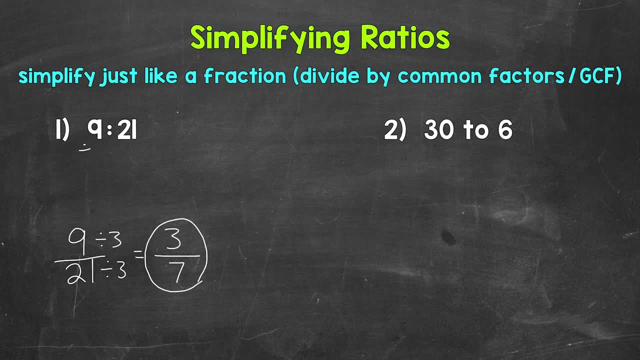 아까 말했다. you can take the fraction form of your simplified ratio and rely on the colon and rewrite it. So the power factor Four and four make up this equationール. As I've told you, you can separate it by Boomstack, at least by removing 2 to inteiro giờ, the half-life ratio. 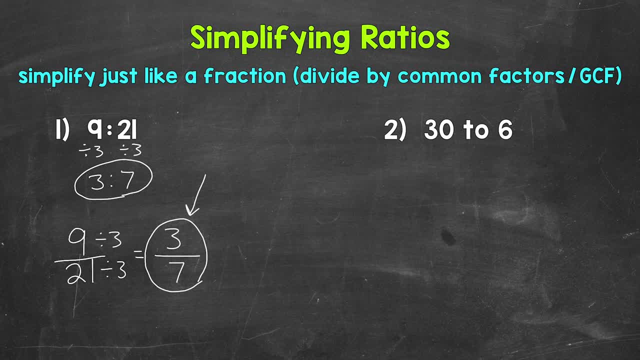 or by integrating with the negative two, For substituting it with a colon, you integrate both. sleep and gång put together, and so it should put together all your Utensilsczumuska solid, and So divide by three, by three and three, and we get all that way as well. Now we can also take the fractional. 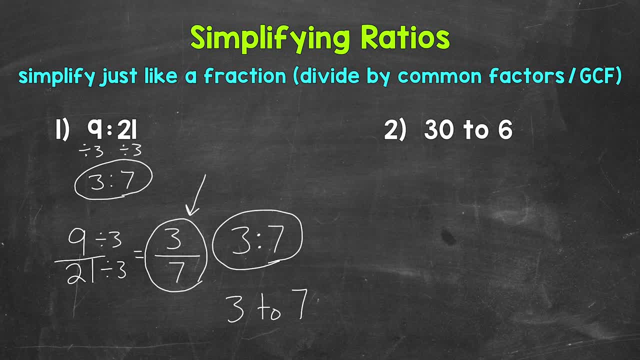 form of our simplified ratio and rewrite it using a colon: three to seven or using the word to all of those to 7, or 3 to 7.. Let's move on to number 2, where we have 30 to 6.. I'll rewrite this ratio as a. 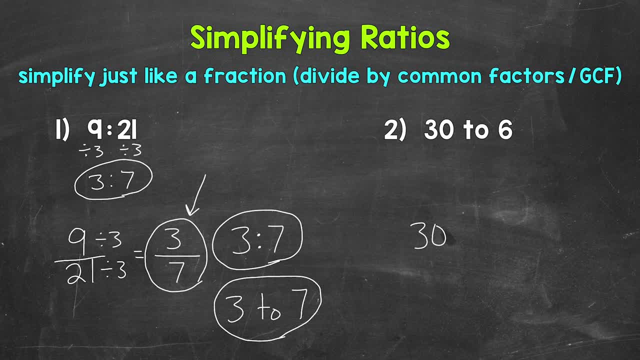 fraction as well. So 30 to 6.. Now we need to think of common factors between 30 and 6.. I'm going to start by using the greatest common factor and simplify this ratio in one step. Then we'll take a look at what it looks like to simplify in multiple steps. So the greatest common factor. 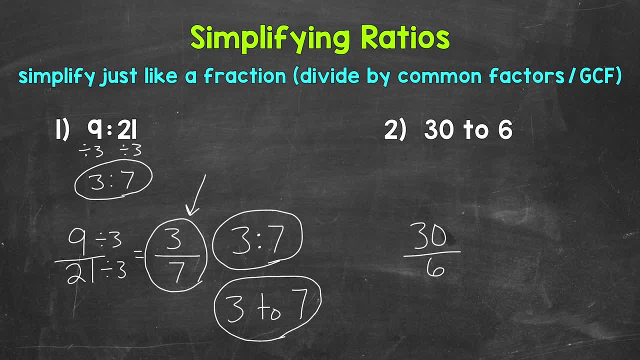 step. then we'll take a look at what it looks like to simplify in multiple steps. so the greatest common factor between 30 and 6 is 6. so let's divide both of these by 6. 30 divided by 6 is 5. 6 divided by 6 is 1. the greatest common factor between: 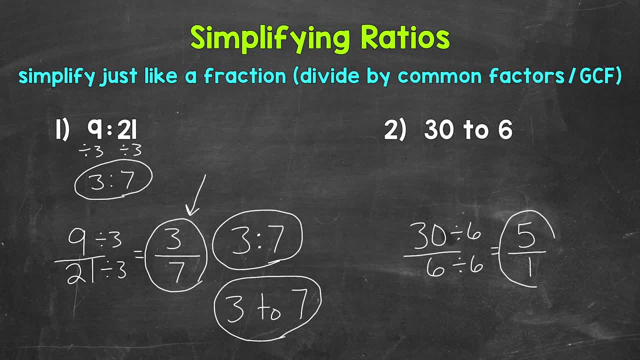 5 and 1 is 1. so this is our simplified ratio: 5, 2, 1. now that is an improper fraction, but we want to leave it as an improper fraction because this is a ratio. a ratio compares and shows the relationship between two quantities or numbers. so again, let's leave it as an. 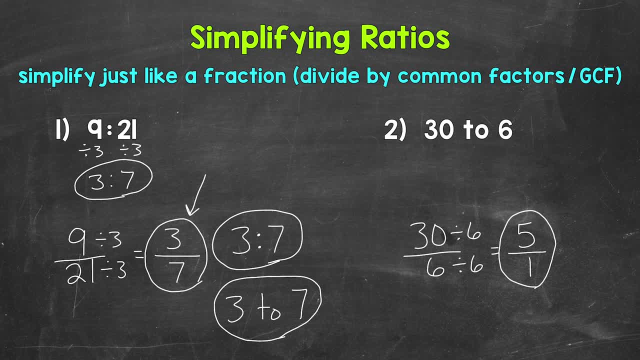 improper fraction. so we have those two numbers that are being compared. so now we're going to go through a different path that we can simplify this ratio. let me rewrite that: 30 to 6.. So we're not going to use the greatest common factor of 6. We're actually going to start. 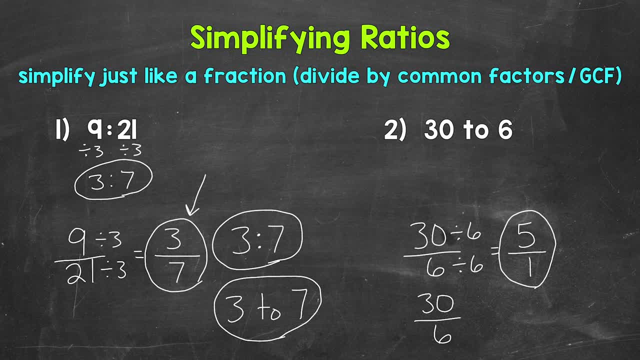 with 2.. 2 is a common factor between 30 and 6.. So let's divide 30 by 2 and 6 by 2.. 30 divided by 2 is 15.. 6 divided by 2 is 3.. So we got 15 to 3, which is different than 5 to 1.. Well, that's. 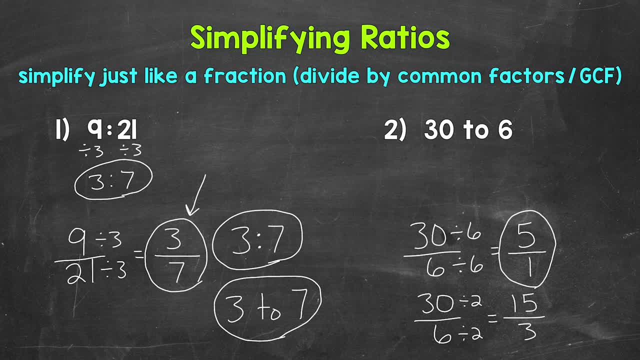 because we still have other common factors other than 1, that we can divide 15 and 3 by here. to further simplify this, to further break this down: Well, 3 is a common factor between 15 and 3.. So let's divide 15 by 3.. 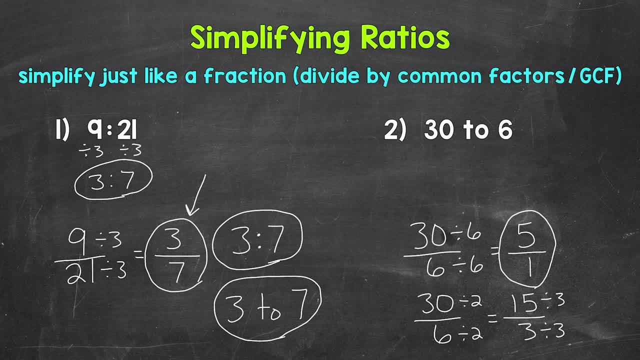 15 divided by 3 is 5.. 3 divided by 3 is 1.. So we ended up with 5 to 1 that way as well. So keep in mind that there can be multiple paths to simplifying a ratio, just like when we simplify. 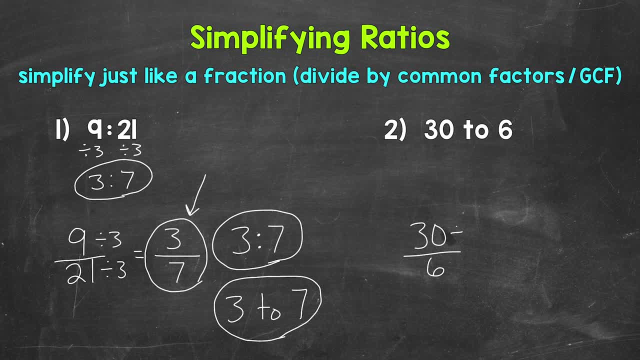 between 30 and 6 is 6.. So let's divide both of these by 6.. 30 divided by 6 is 5.. 6 divided by 6 is 1.. The greatest common factor between 5 and 1 is 1.. So this is our simplified ratio. 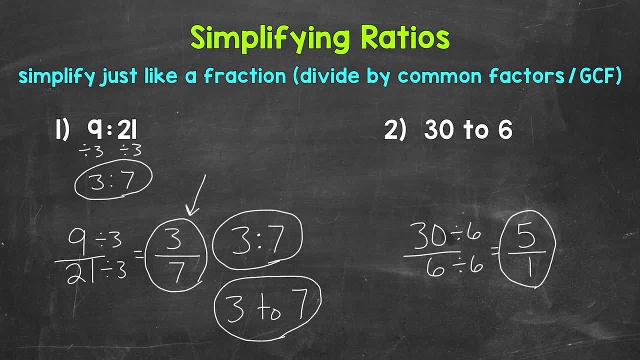 5. Now, that is an improper fraction, but we want to leave it as an improper fraction because this is a ratio. A ratio compares and shows the relationship between two quantities or numbers. So again, let's leave it as an improper fraction. So we have those two numbers that are being 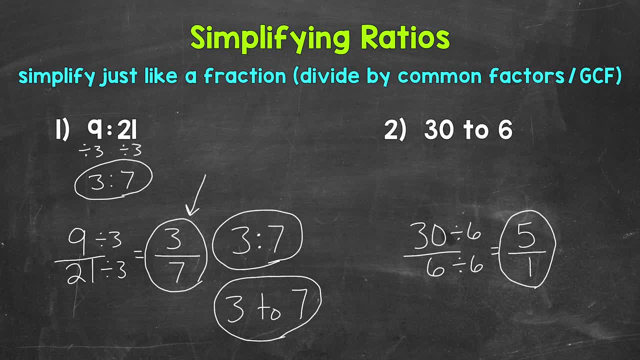 compared. So now we're going to go through a different path that we can simplify this ratio. Let me rewrite 30 to 6.. So we're not going to use the greatest common factor of 6. We're actually going to start with. 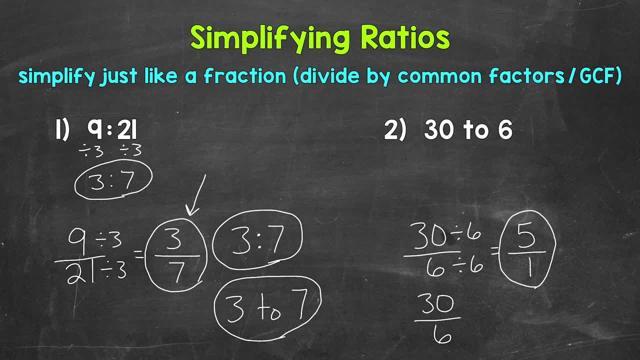 2.. 2 is a common factor between 30 and 6.. So let's divide 30 by 2 and 6 by 2.. 30 divided by 2 is 15.. 6 divided by 2 is 3.. So we got 15 to 3, which is different than 5 to 1.. Well, that's because we 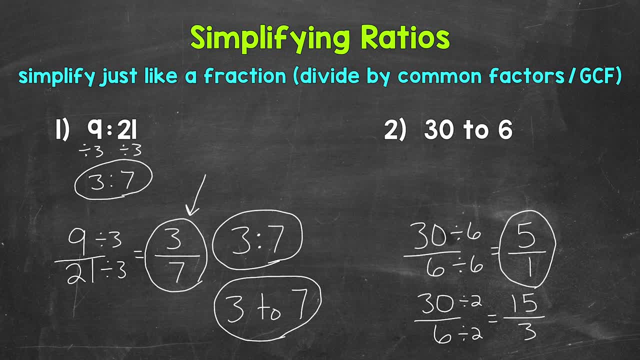 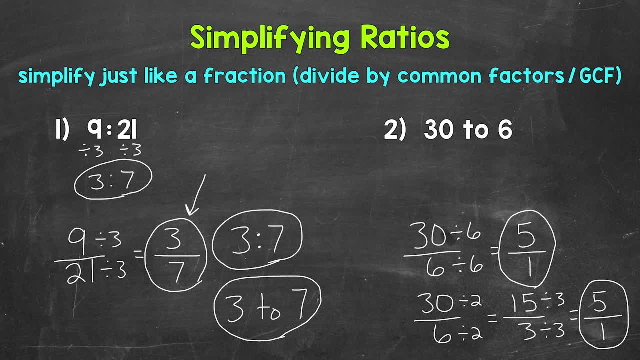 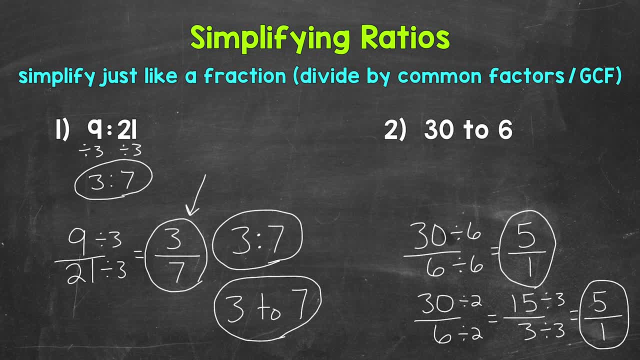 ratio, just like when we simplify fractions- And again we can simplify from that original form- Let's divide by 6 up here as well. So 30 divided by 6 and 6 divided by 6.. That gives us 5 to 1.. 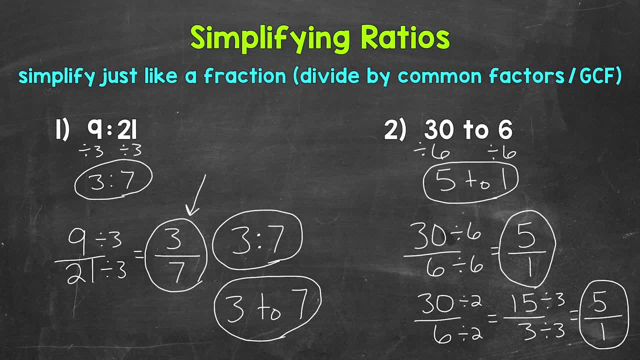 And again, we can always rewrite Our ratio in the form that we would like. So, for example, we can take our fractional form and rewrite this using a colon, So 5 to 1, or using the word 2.. All of those ratios mean. 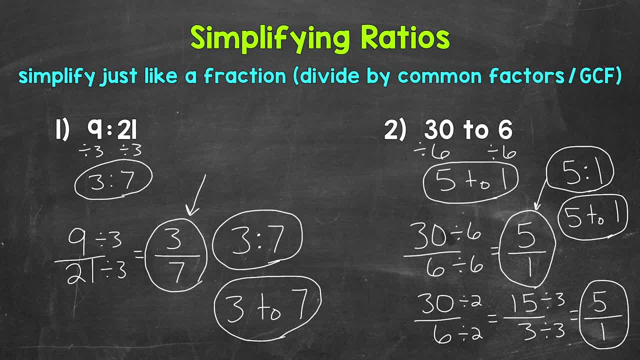 the same thing: 5 to 1.. Now I do want to mention one more thing, and that's that a ratio can be in simplest form from the start. If the greatest common factor between the terms of a ratio is 1, then it's already in simplest form And you can't do any more simplifying. So that's something to 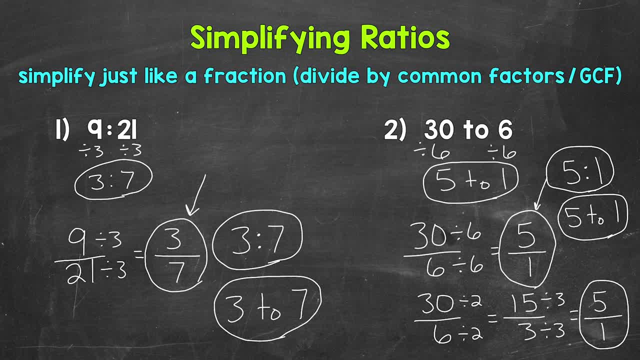 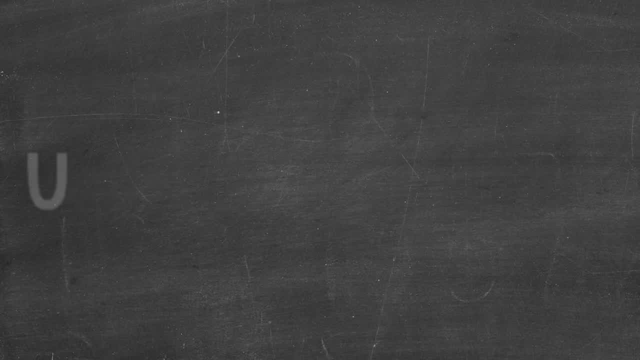 keep in mind. So there you have it. There's how you simplify ratios. I hope that helped. Thanks so much for watching. Until next time, peace.